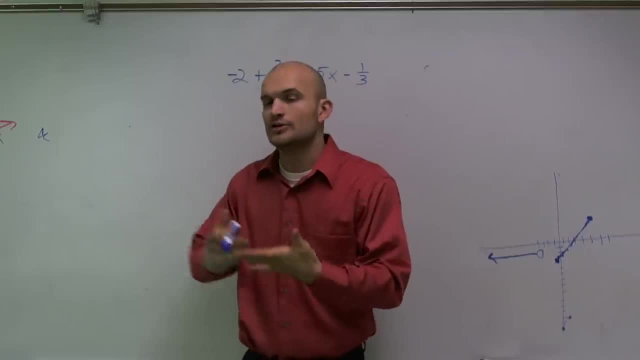 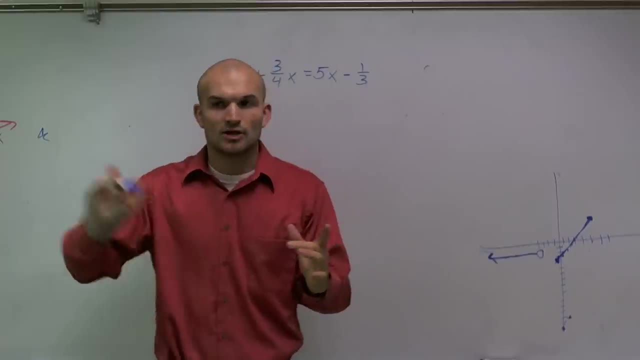 divided by four. So to undo division, we do multiplication right, Because think about it this way. You know a number, let's say eight, eight divided by two, and then multiply by two. Well, eight divided by two is four. Four multiplied by two gives you back eight. So 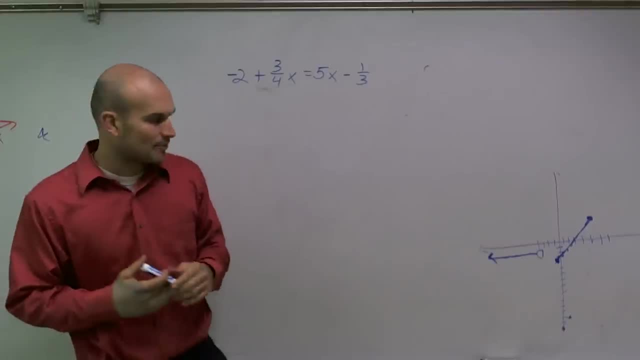 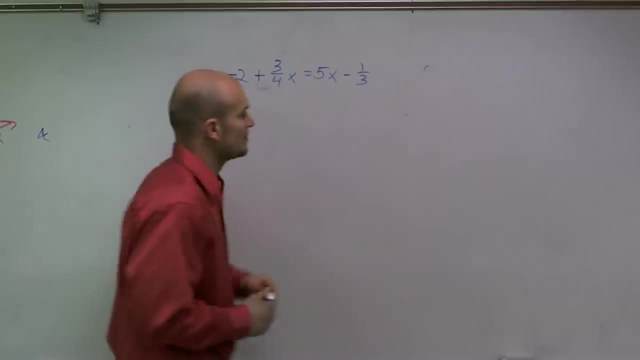 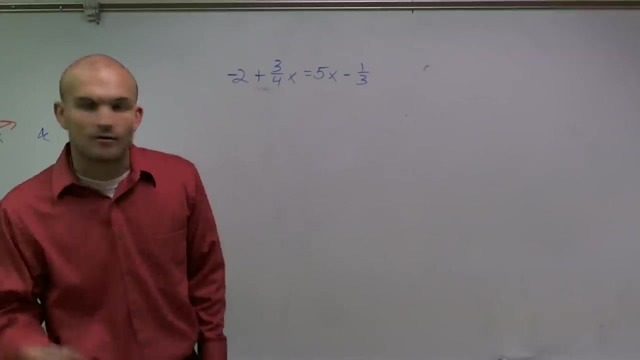 they undo each other what we call inverse operations. So if I can take what I'm divided by and multiply by those numbers, I can get rid of them. So the question is: I'm divided by four, So to undo divided by four, I have to multiply by four And you undo division. 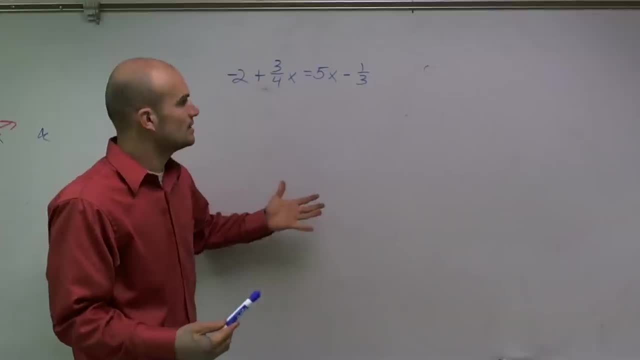 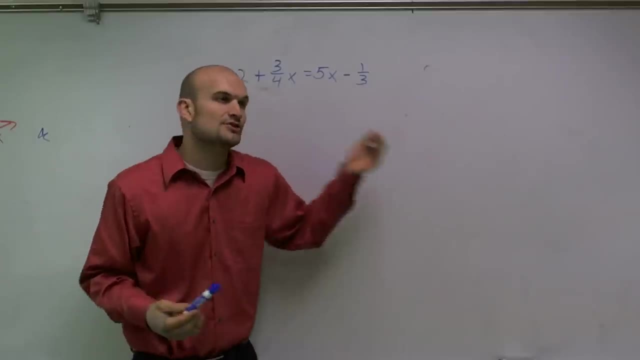 by three. I have to multiply by three. Well, which one do you choose? And because, remember, it's an equation- you can't multiply by four on this side and then multiply by three on this side, because whatever you do on one side of the equation, you have to do the same on the other. 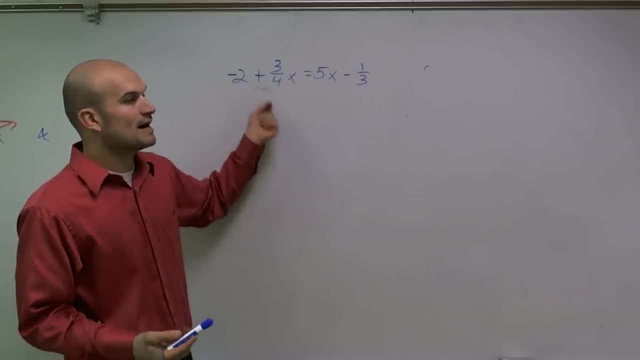 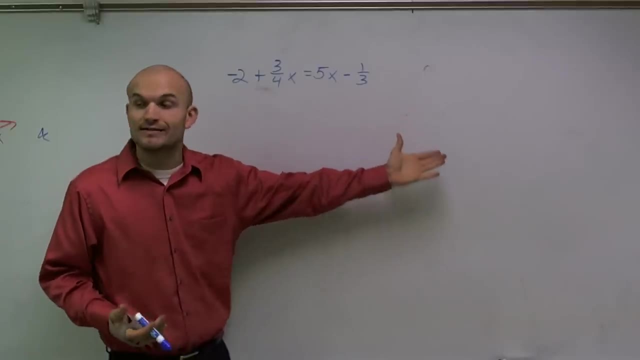 side of the equation. So the correct answer is: I have to multiply by three and I have to multiply by four, by every single term. Because it's an equation, you have to make sure you treat everything equally. So when you multiply by three and you multiply by four, well, that's the same. 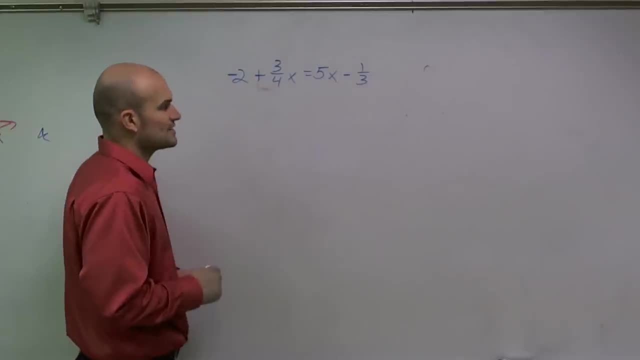 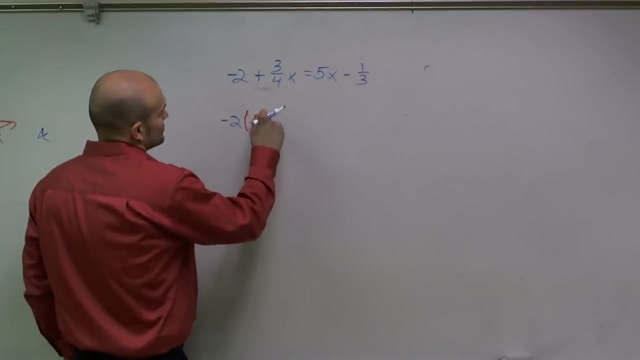 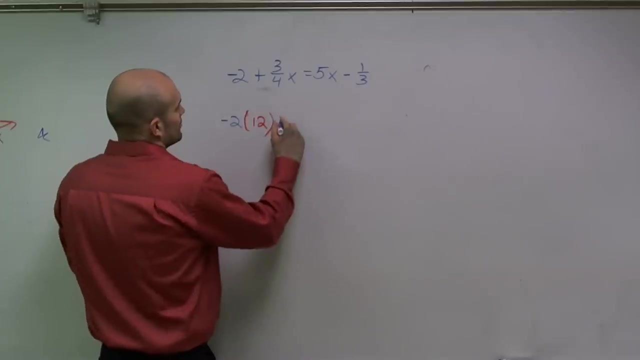 as multiplying by 12, right, Because three times four is 12.. So to clear fractions for this problem I'm going to have to multiply everything times 12.. So I'll do negative two times, not negative 12, 12 plus three-fourths x times. 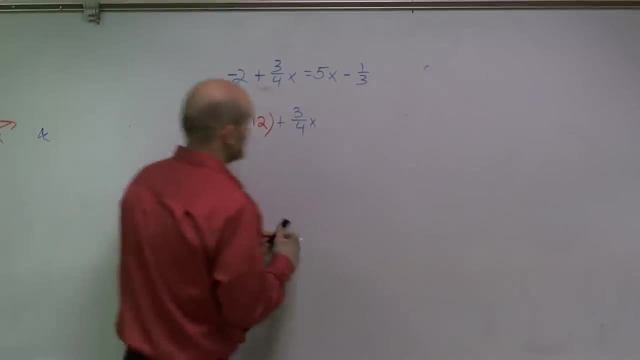 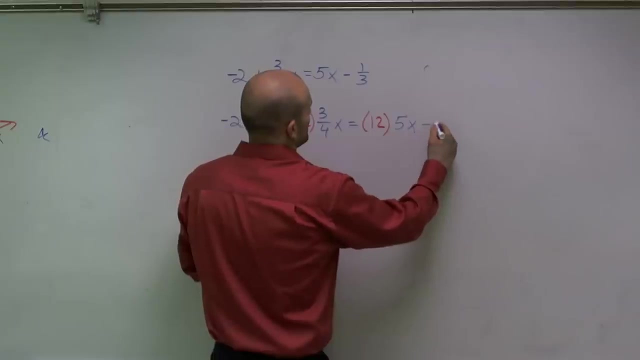 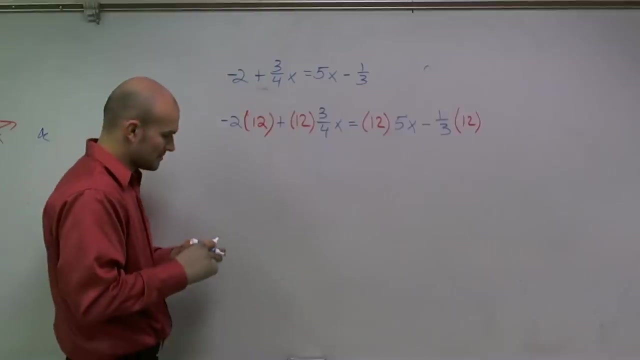 ah, Let's write that in front, It'll help us out. Times 12 times three-fourths x equals 12 times five x minus one-third times 12.. All right, So let's go through this: Negative two times negative 12, negative 24.. 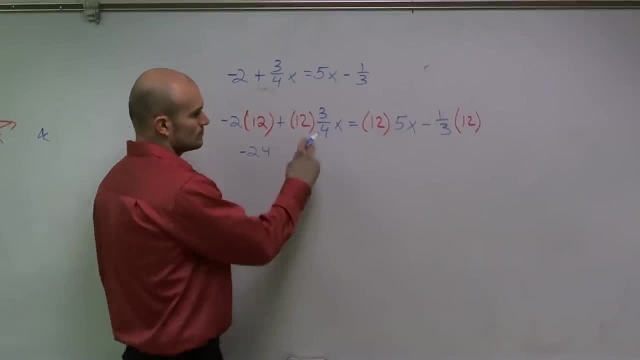 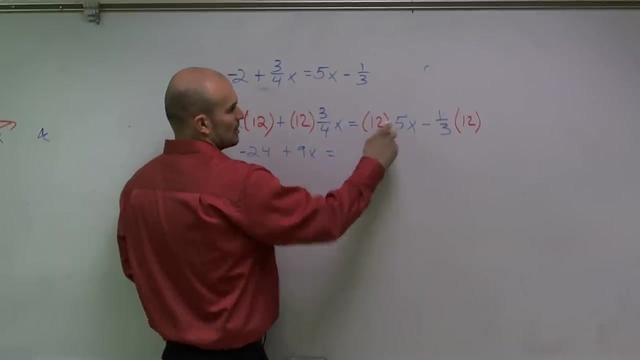 12 times three-fourths. There's a couple ways to do this. You can divide first and then multiply, or multiply then divide. 12 times three is 36.. 36 divided by four is nine. 12 divided by four is three. Three times three is nine. So either way, you're going to get nine x equals 12 times five. 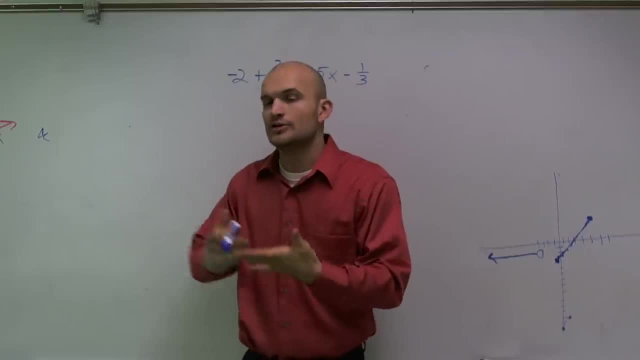 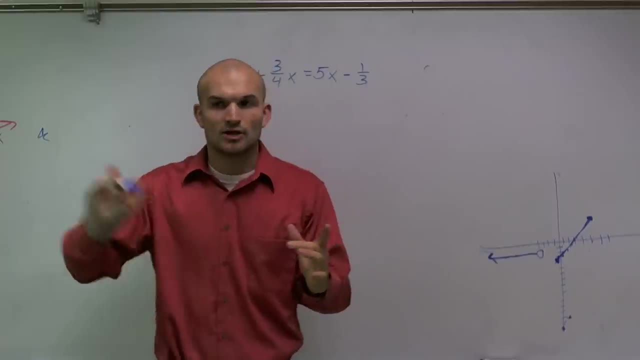 divided by four. So to undo division, we do multiplication right, Because think about it this way. You know a number, let's say eight, eight divided by two, and then multiply by two. Well, eight divided by two is four. Four multiplied by two gives you back eight. So 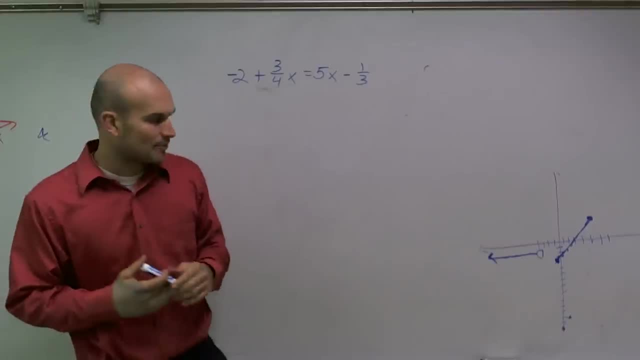 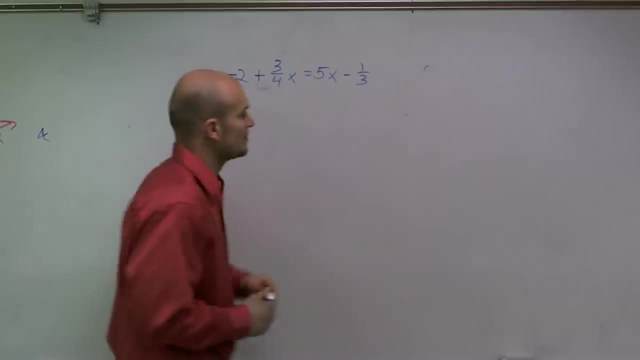 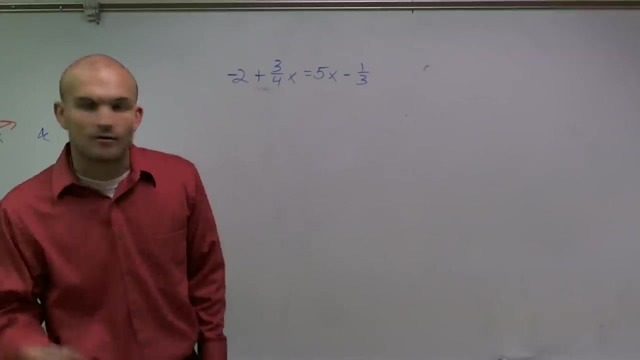 they undo each other what we call inverse operations. So if I can take what I'm divided by and multiply by those numbers, I can get rid of them. So the question is: I'm divided by four, So to undo divided by four, I have to multiply by four And you undo division. 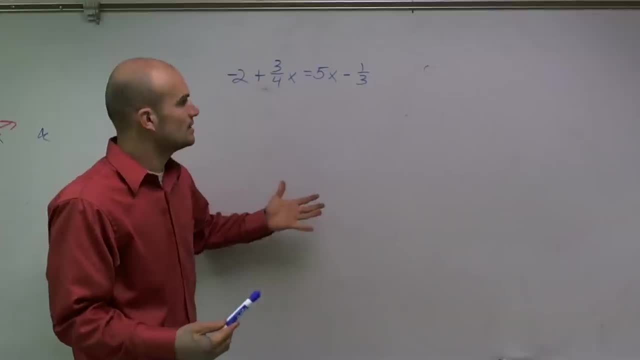 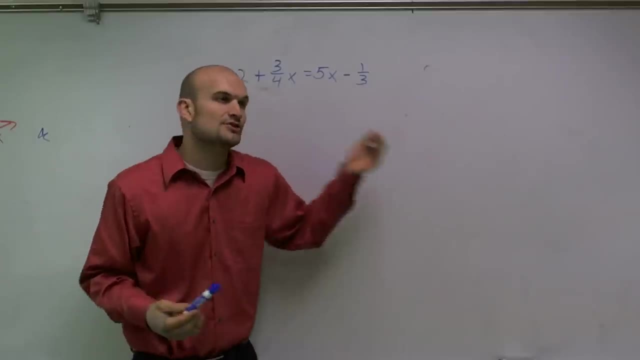 by three. I have to multiply by three. Well, which one do you choose? And because, remember, it's an equation- you can't multiply by four on this side and then multiply by three on this side, because whatever you do on one side of the equation, you have to do the same on the other. 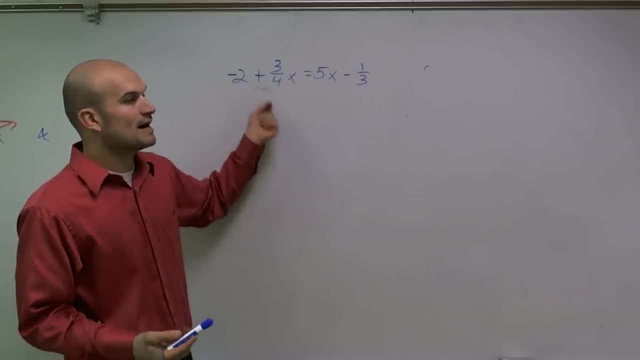 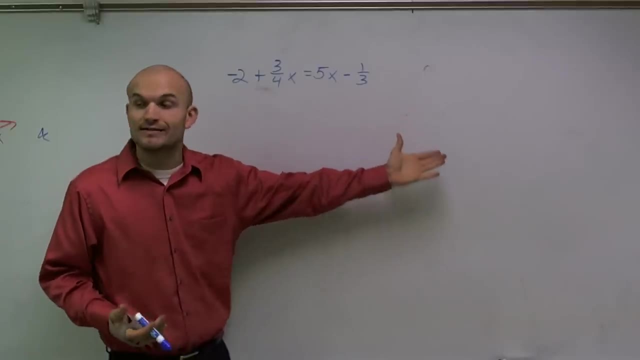 side of the equation. So the correct answer is: I have to multiply by three and I have to multiply by four, by every single term. Because it's an equation, you have to make sure you treat everything equally. So when you multiply by three and you multiply by four, well, that's the same. 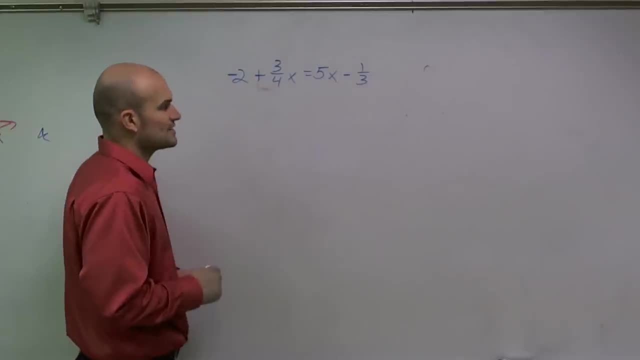 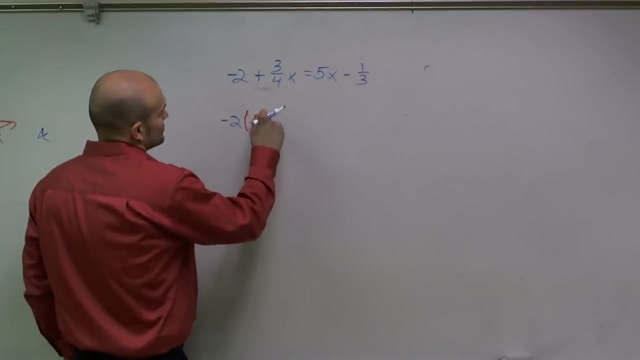 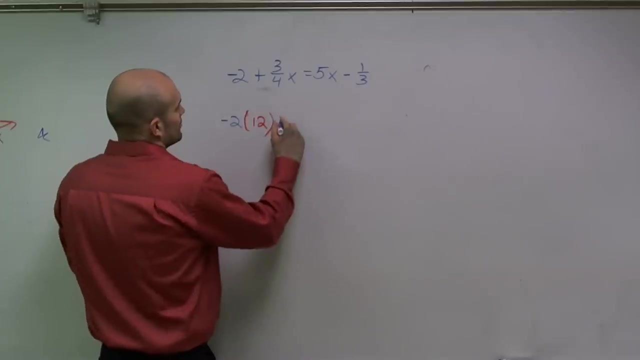 as multiplying by 12, right, Because three times four is 12.. So to clear fractions for this problem I'm going to have to multiply everything times 12.. So I'll do negative two times, not negative 12, 12 plus three-fourths x times. 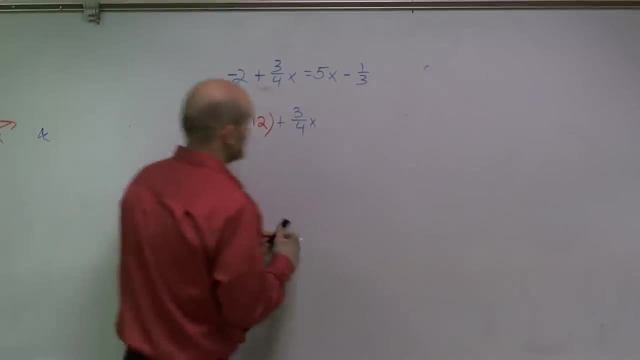 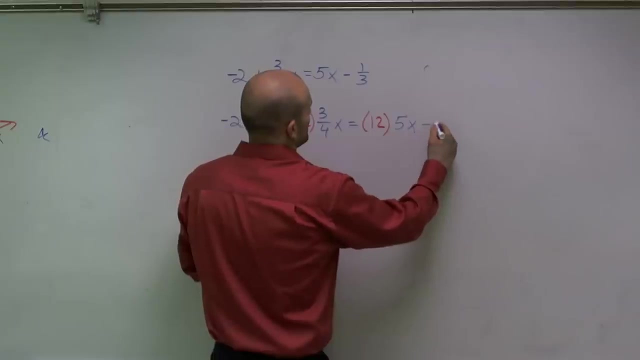 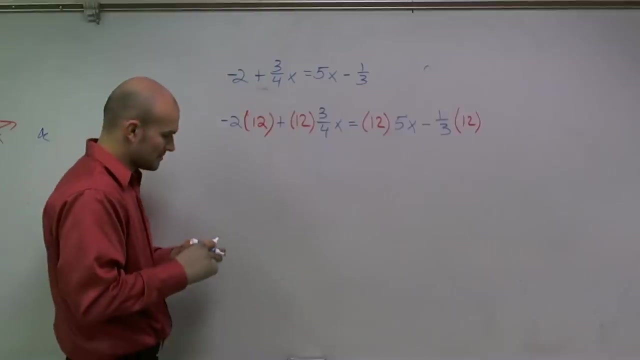 ah, Let's write that in front, It'll help us out. Times 12 times three-fourths x equals 12 times five x minus one-third times 12.. All right, So let's go through this: Negative two times negative 12, negative 24.. 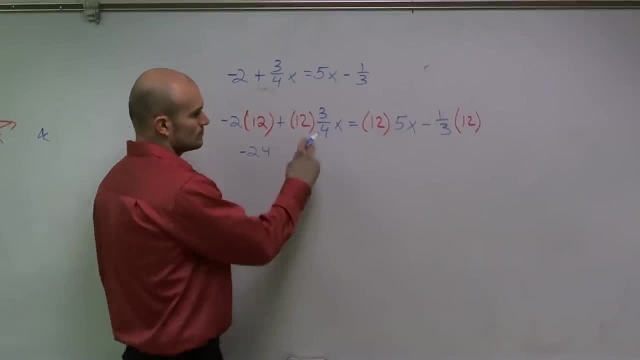 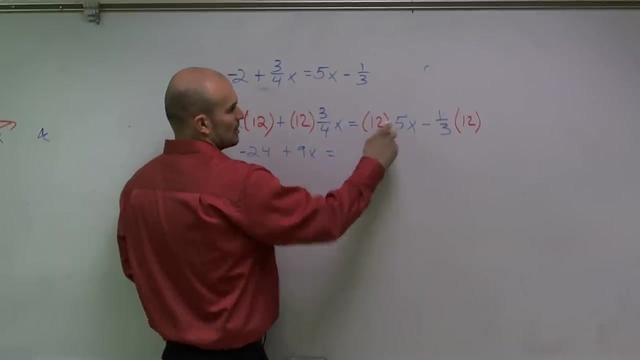 12 times three-fourths. There's a couple ways to do this. You can divide first and then multiply, or multiply then divide. 12 times three is 36.. 36 divided by four is nine. 12 divided by four is three. Three times three is nine. So either way, you're going to get nine x equals 12 times five.